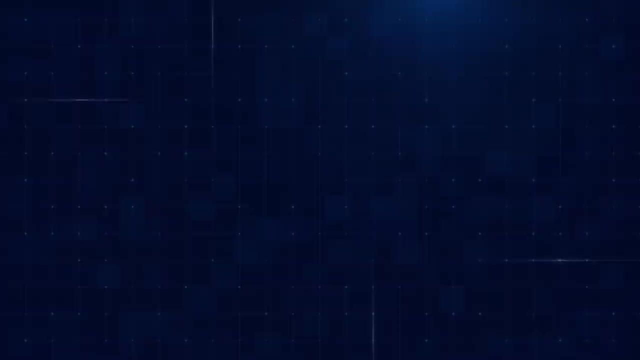 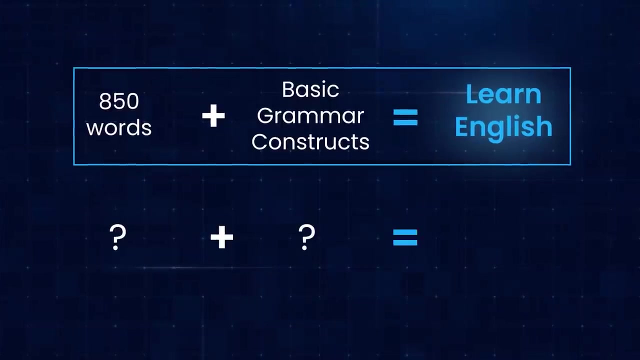 and pronunciation to the non-native speakers and was a huge success. But how could just 850 words and a few basic grammar constructs help people learn English, And can we use the same principles to learn a new programming language? To answer that, we need to know a few. 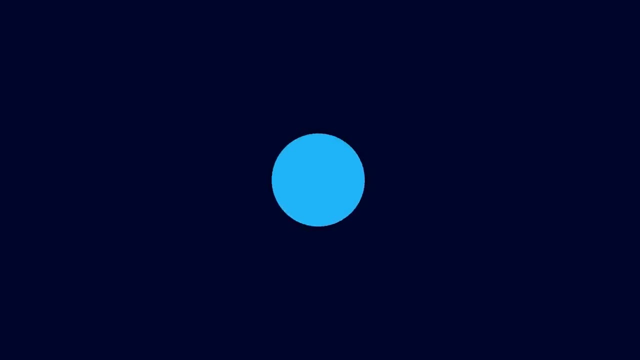 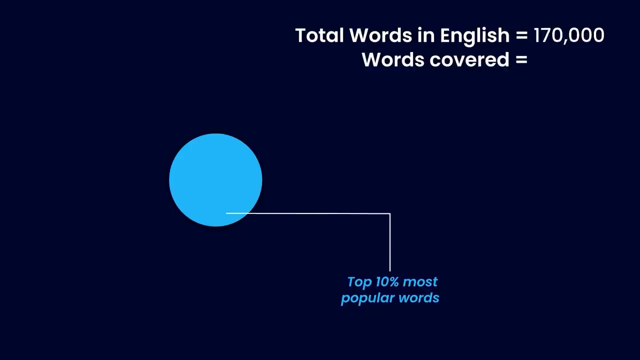 things about how the languages exactly work. Imagine a circle that contains top 10% most popular words Among the 170,000 total words. in English, this circle contains words like I, me, you, eat, drink, etc. And then we have another circle around it that contains the next 10% most popular words. 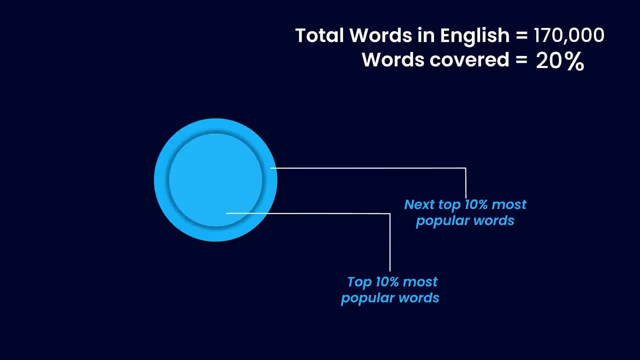 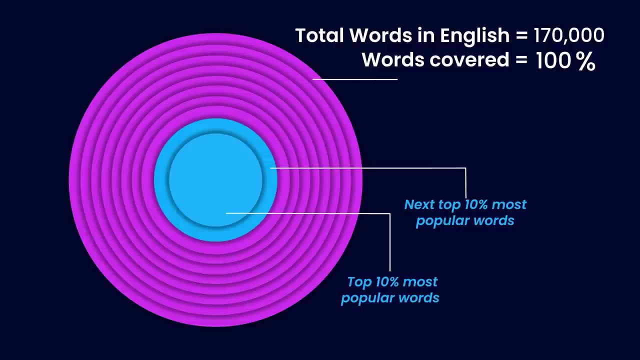 This would contain words like overpaid and programmer, which makes sense. And we can keep making these 10% circles until we cover all 170,000 words. In case you are curious, the outermost circle contains words like nincompoop and teetotaler. For simplicity, let's combine the: 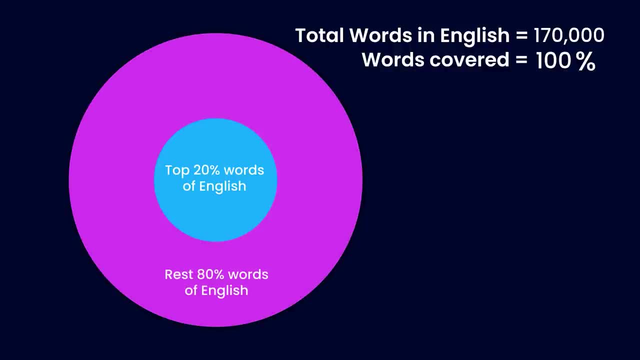 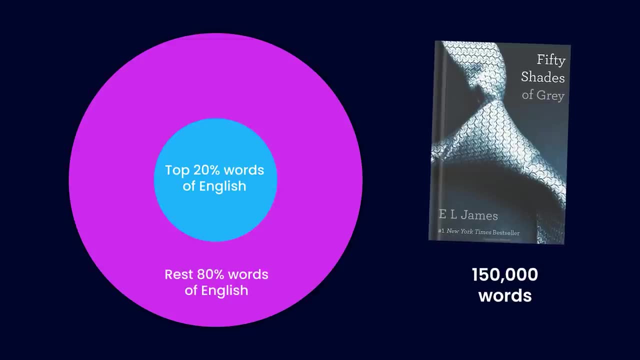 two circles together and the rest of the circles together. Now imagine that you start reading one of the best novels of our time called Fifty Shades of Grey, which has a total of 150,000 words. What you'll find is that 80% of these 150,000 words in the book come from the inner circle. 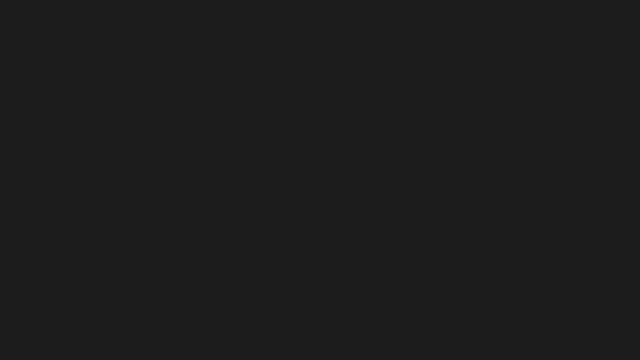 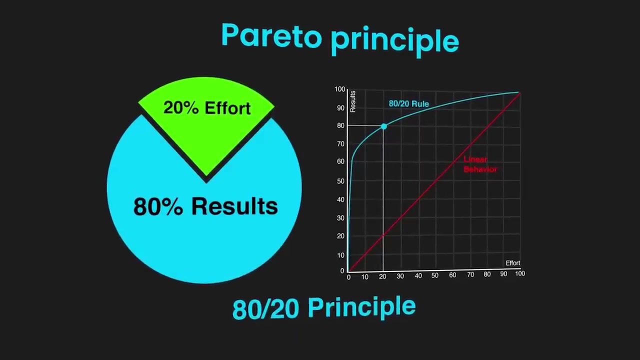 and the rest of the 20% words lie in the outer circle. For those who don't know, this is also called Pareto Principle. Pareto Principle states that 20% of your effort results in 80% of your outcomes, And this is a very powerful principle, This powerful principle. 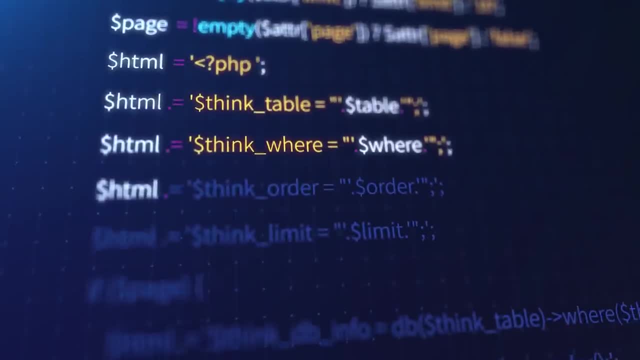 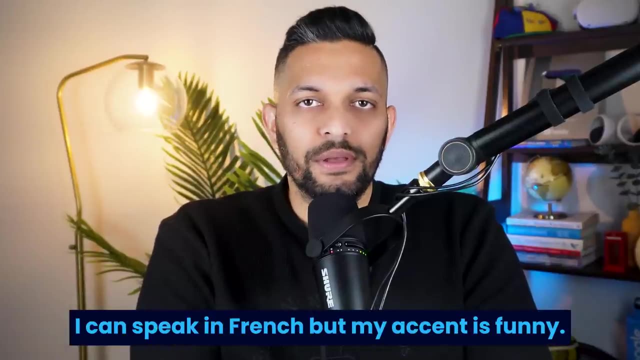 is the main idea behind the basic English, as well as learning any new programming language really fast. I applied the same principle to learn French, and now je peux parler en français, mais mon accent est marron. Learning a new spoken language is one thing, but learning a language. 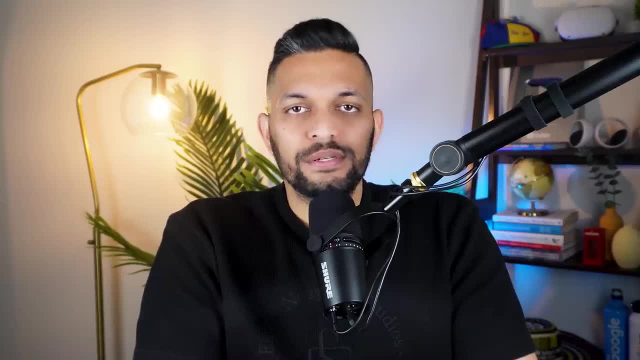 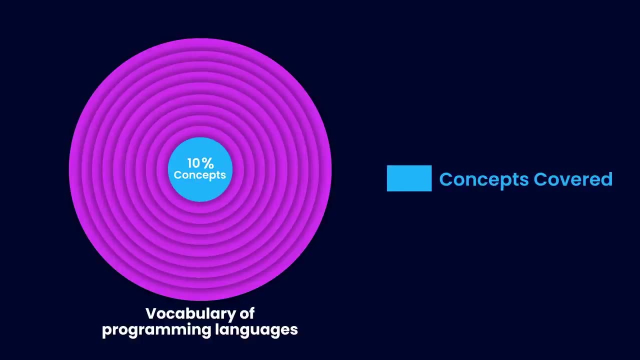 that computer understands is totally different. Well, that's not true. Let's build the same 10% circles for the vocabulary of a programming language. What would be the top 10% most popular concepts here? I believe it would include different data types like int, float, string. 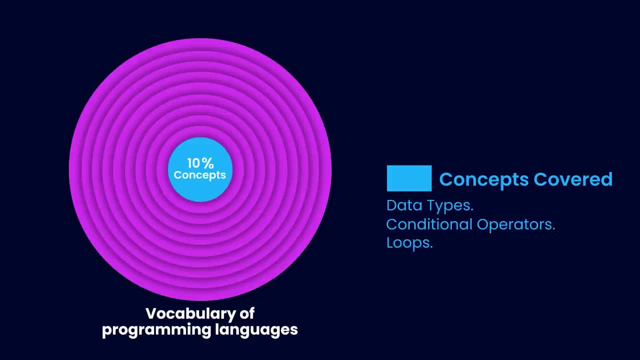 or array, etc. Maybe if-else statements and for-loops would also be part of this circle. Maybe writing functions and classes would also be here. If you move outside to the next circle, you might have concepts like polymorphism and inheritance etc. And you can keep drawing these. 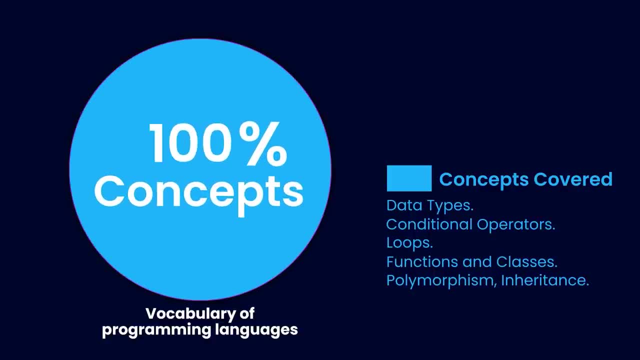 circles until you reach the outermost circle that might contain some very specialized libraries. Now, if you pick all the GitHub repos in the language of your choice, what you'll find is that 80% of the code would come from this inner 20% circle. And, following what we learned from basic, 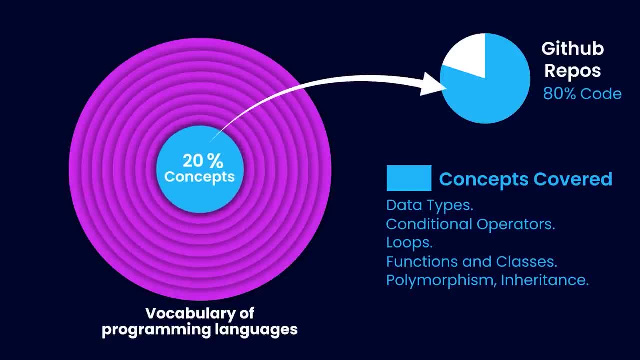 English examples, we'll be able to see that 80% of the code would come from this inner 20% circle, For example. we'll focus on this 20% circle first, But as we do this, we need to be careful about two. 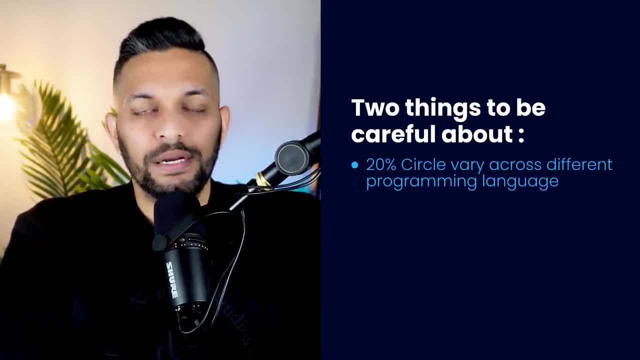 things. Number one: this 20% circle might vary a little bit depending on the language you choose. For example, in Java you might have array list, but we'll call it just list. in Python Or in JavaScript, you might have async of it, which might be very different from other languages. 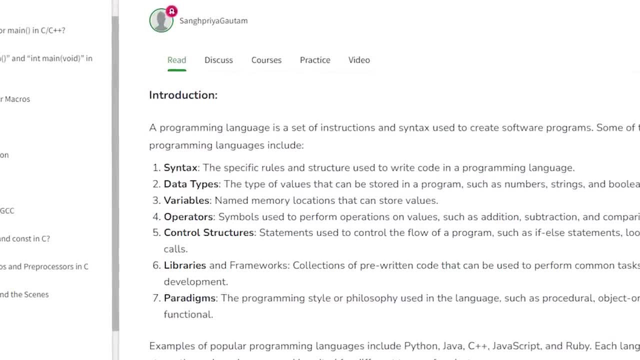 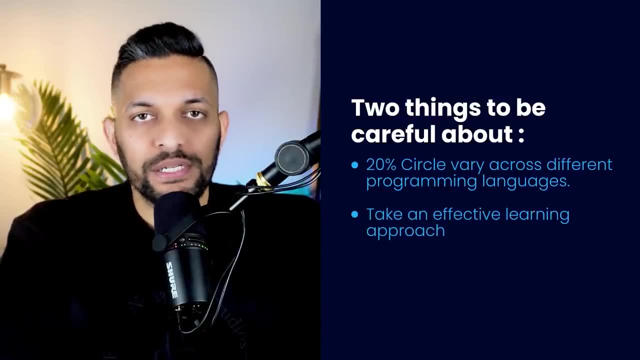 The point is, the top 20% circle might vary and you would want to do your own research to find the top concepts in the language of your choice. Number two: when you're learning these concepts, you need to change your method of learning If you are trying to learn a new spoken. 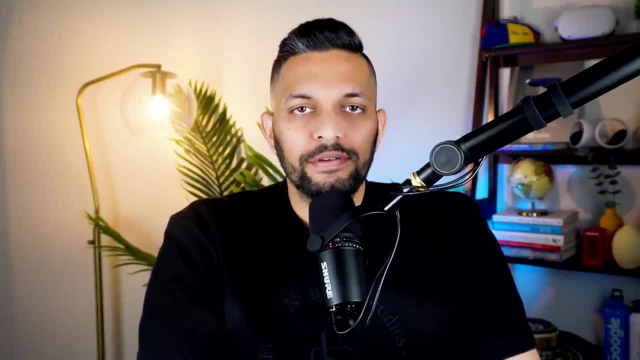 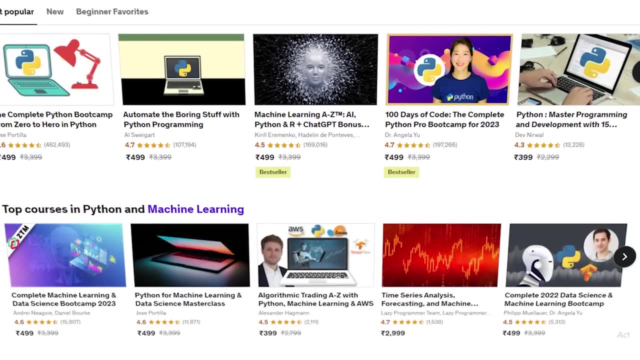 language. let's say French, for example. no matter how many movies or TV series you watch in French, you will not be able to speak in French unless you actually try to talk in French. In the same way, no matter how many lectures or video tutorials you watch in Python, you will not be able to learn. 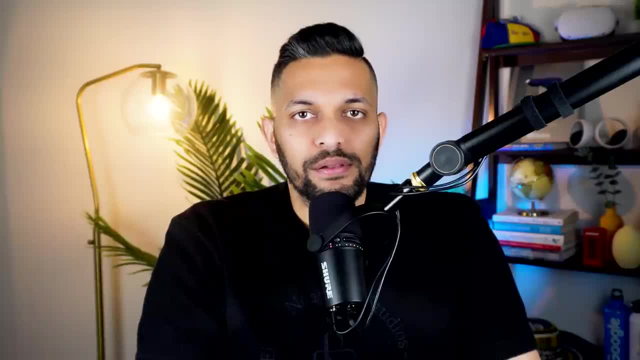 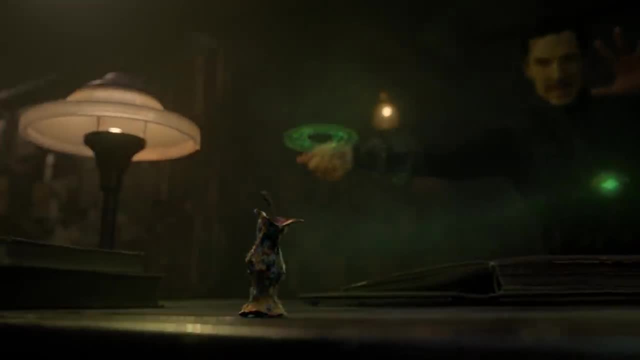 Python. unless you actually try to code in Python In a video tutorial, you usually get the code that already works, and if you copy it, sure enough it will work for you as well. But programming is the art of breaking and fixing things. That's why I recommend interactive learning instead of casual. 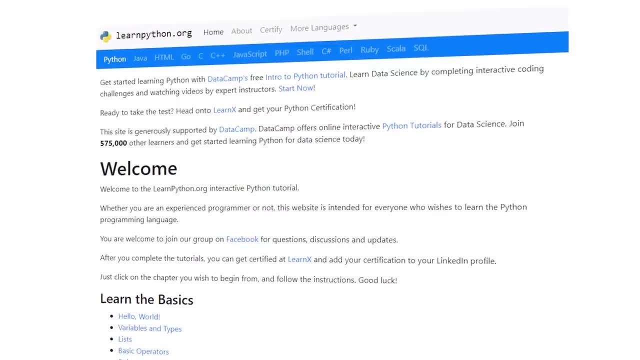 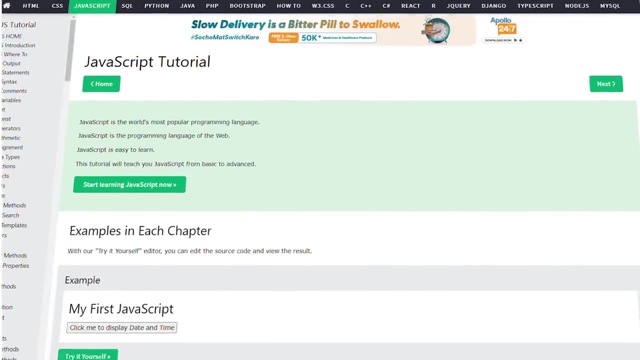 learning. For example, if you want to learn Python, you can go to learnpythonorg and do exercises, break things and fix them as you learn new concepts. Similarly, for JavaScript, you can go to W3Schools. I'm sure you can find this kind of platform in other languages as well. 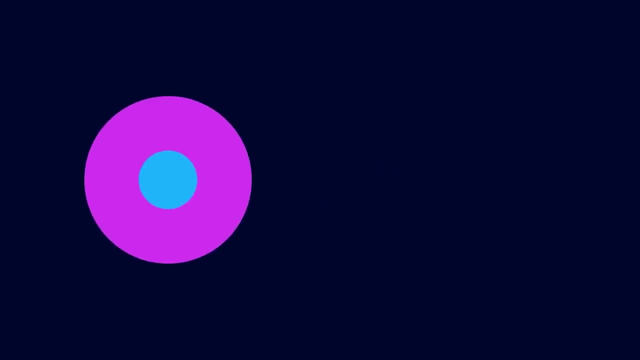 Now that you know what to learn and how to learn it, there are two problems left for us to solve: How to remember what we are learning and how to learn the rest of the 80% in the outer circle. To solve the first problem, we need to understand the Ebbinghaus forgetting. 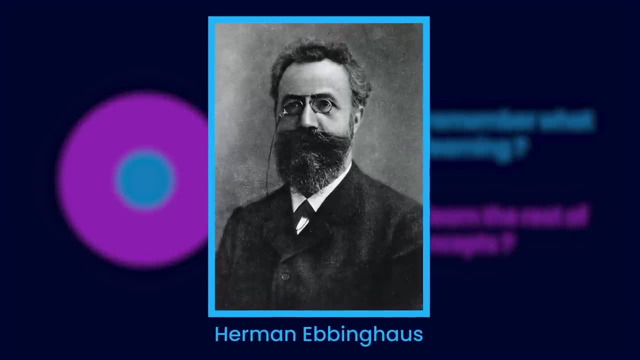 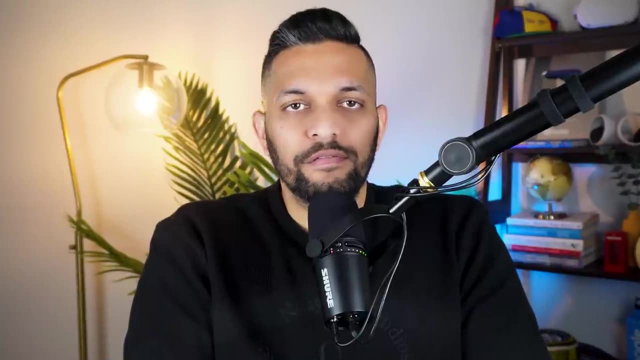 curve. Hermann Ebbinghaus was a German psychologist who is well known for his work on memory and learning. He conducted experiments where he would give himself some nonsense words to remember and then test himself at various intervals to see how many of these words he could actually. 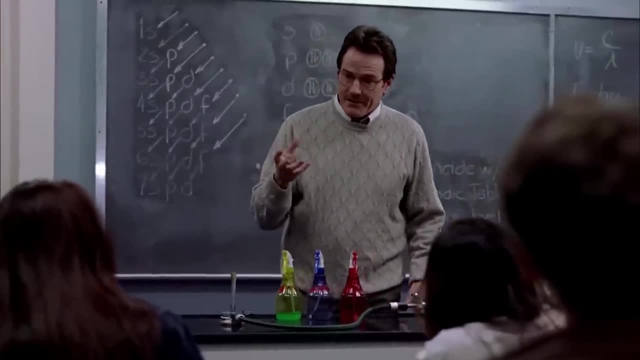 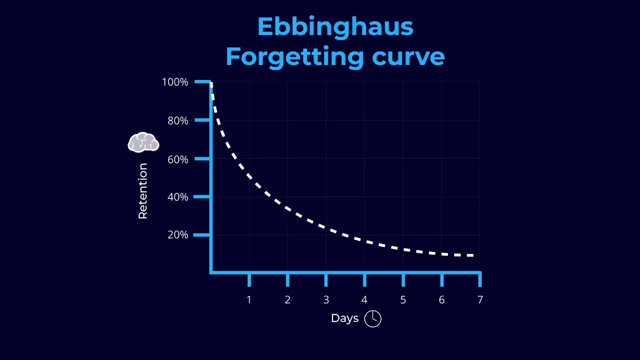 remember. What he found became the backbone of how we teach children in the modern school system. What you are seeing is the famous Ebbinghaus forgetting curve. This graph is a classical exponential decay graph. What this means is that right after we learn something new, we start forgetting it very quickly. The rate of forgetting slows down over. 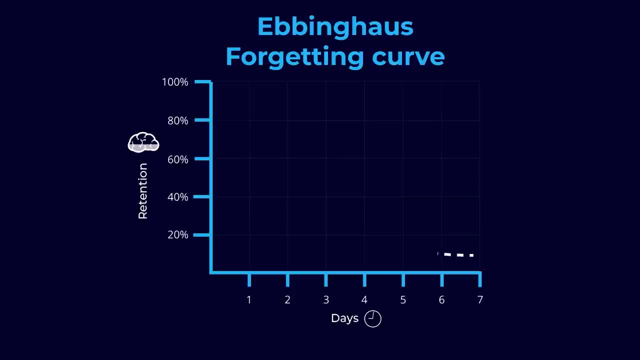 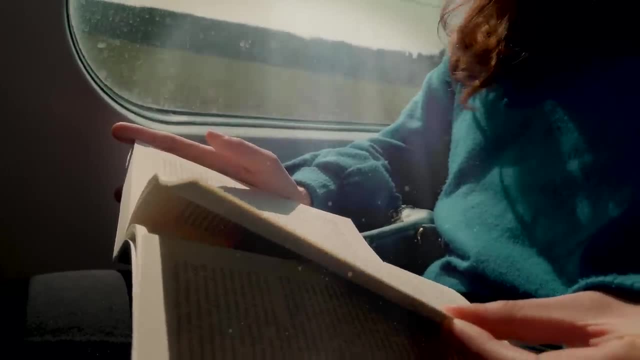 time and in the end we only remember a fraction of what we learned. But what if I told you that there is a way to retain more of what we learned? Ebbinghaus also studied the impact of revision on our retention. What he found was that if you review the words again, you can increase the 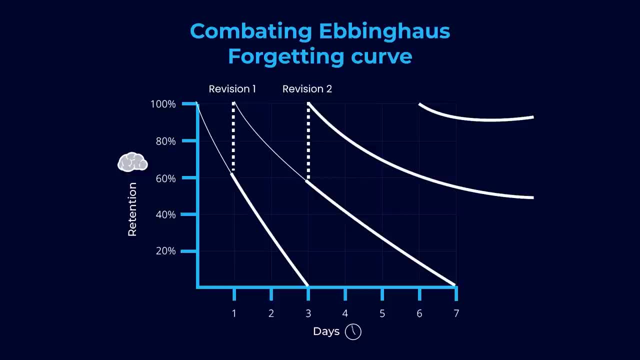 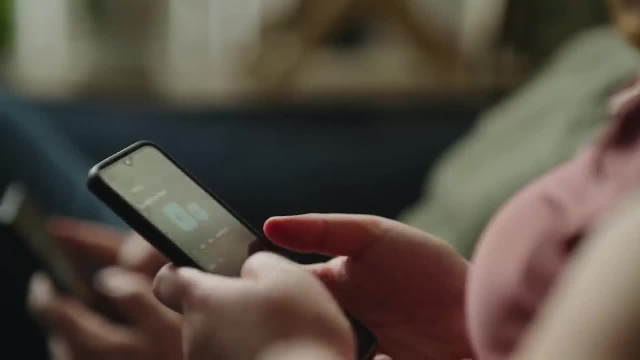 number of words you remember in the end, And if you repeat this multiple times, your retention can keep increasing, And this is called spaced repetition, which many of you might have already heard about. This is the reason why, if you try to learn a new language using an app like Duolingo, they keep repeating the same words again and again. 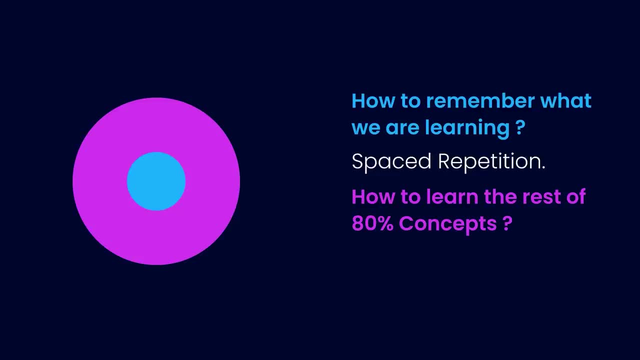 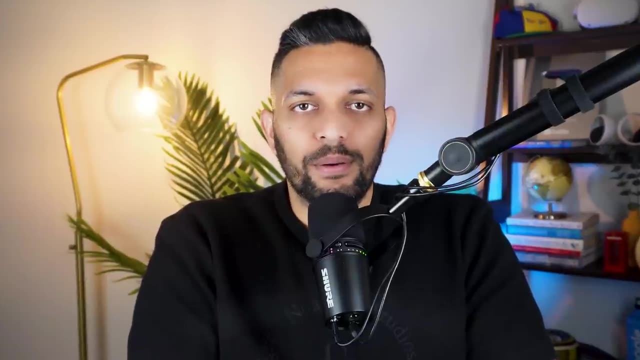 in the exercises, But how do we apply spaced repetition to learning a new programming language? The answer to this question is also the answer to the second problem that we still need to solve. So let's quickly cover the second problem and then we'll talk about the solution. 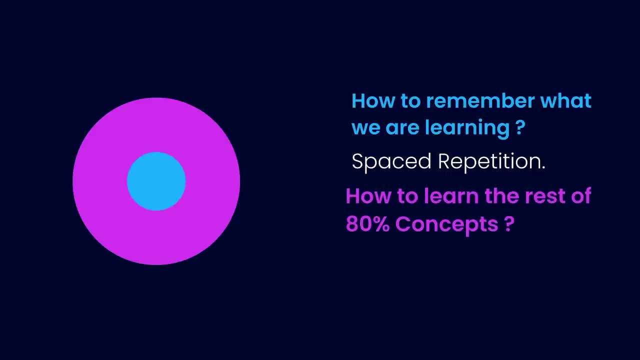 The other pending problem that we have is that we have still not figured out how to learn the remaining 80% of the concepts. For this, we need to take a breath-first approach to our learning. What this means is that, instead of taking some random long, deep path from 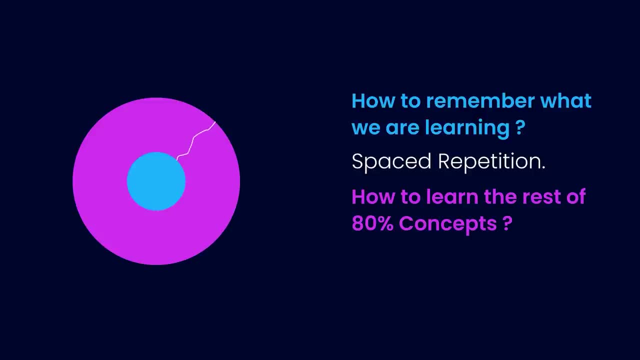 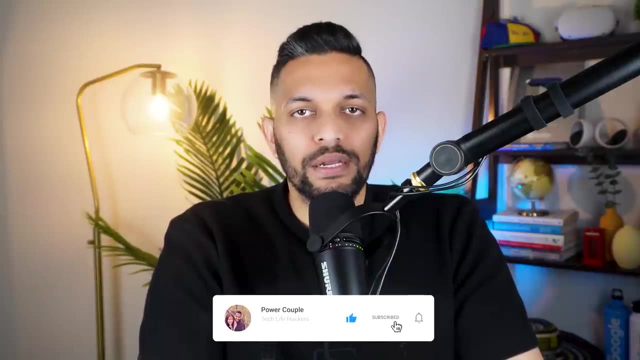 the inner circle to the outer boundary. we just keep enlarging our inner circle. In other words, we slowly keep increasing the breadth of our knowledge. The biggest advantage of doing this is that we are only learning new things that are very close to what we already know. 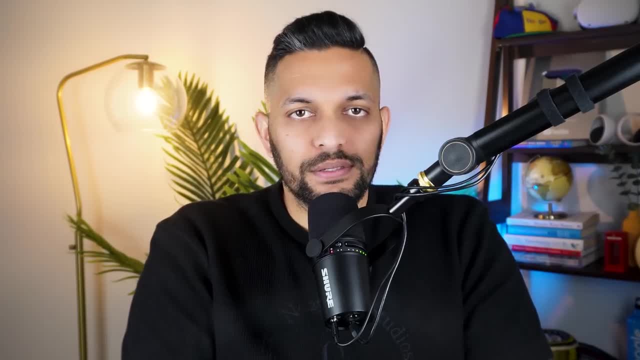 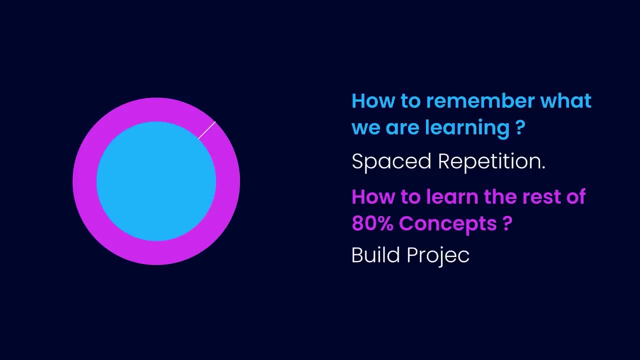 And this makes learning them very easy. But how exactly do we do this? To remember more of what we have learned so far and to learn the remaining 80% concepts, all we need to do is build projects, But not just any projects. 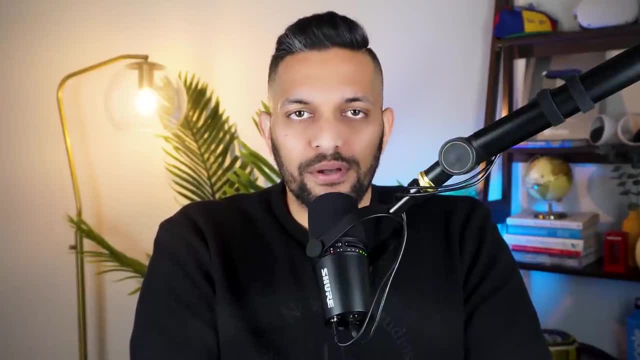 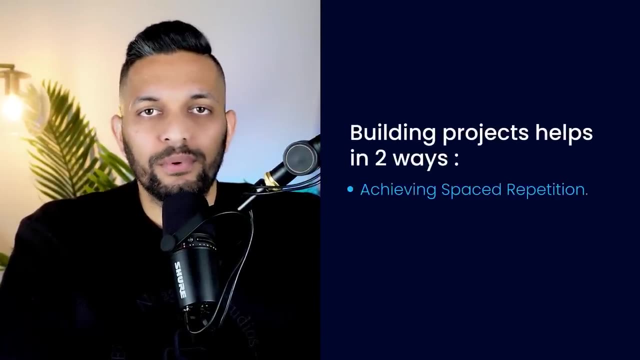 we need projects with increasing difficulty. I'll tell you which exact projects to build in a moment. But building projects helps you in two ways. Number one: when you build projects, you encounter the top 20% concepts again and again, And this helps you achieve spaced repetition. 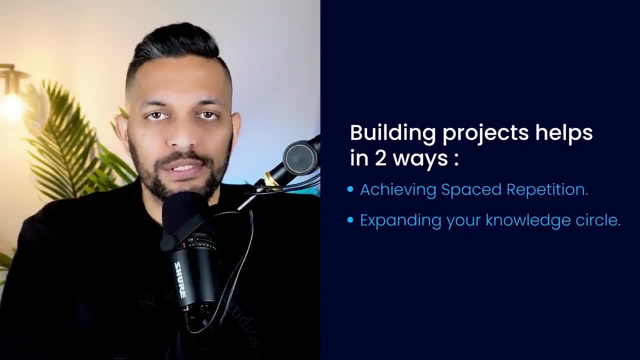 Number two. when you build projects, you will need to learn some new concepts on the go. If you choose your projects carefully and slowly increase the difficulty, you can constantly expand your inner circle to become the same size as the outer circle. One thing to be aware of, though.